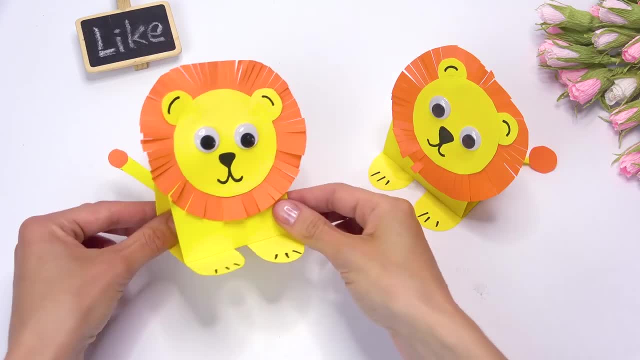 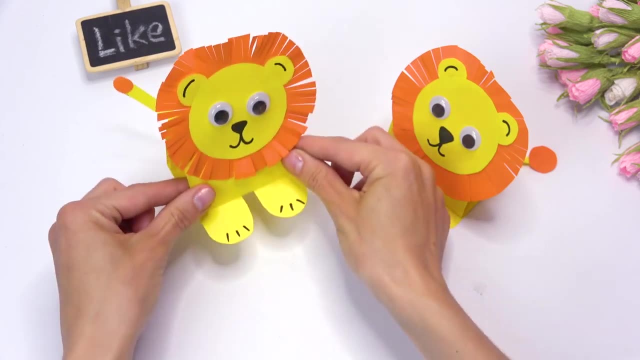 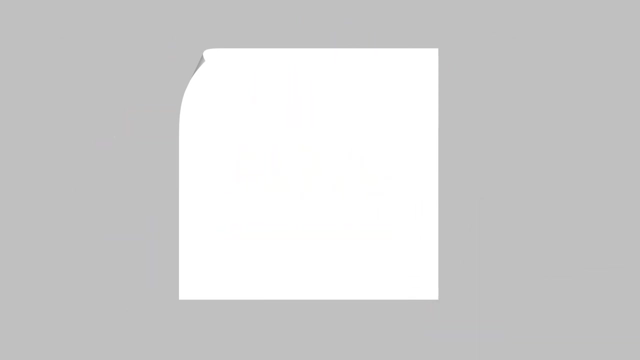 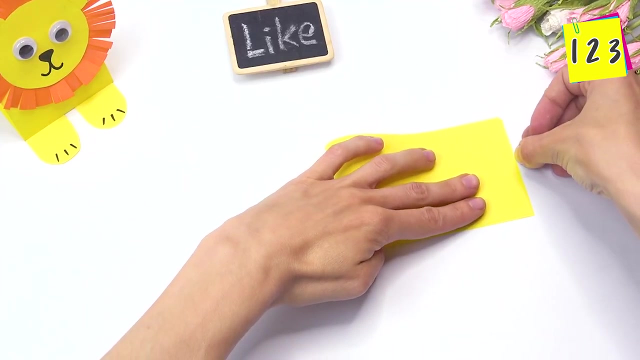 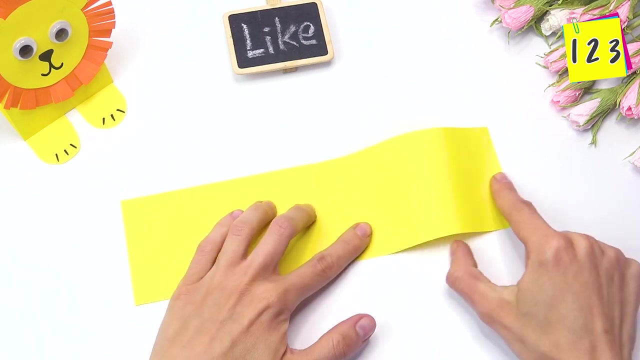 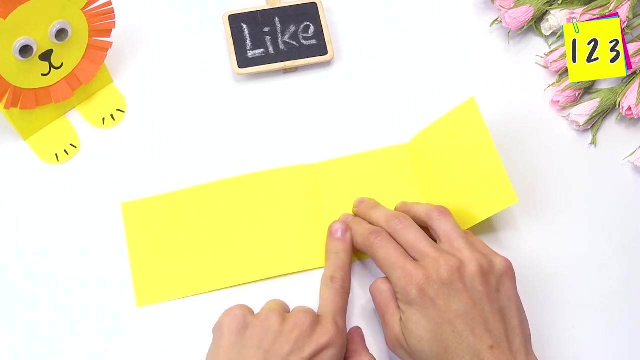 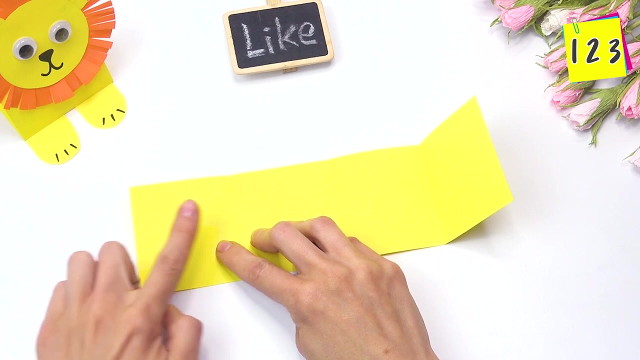 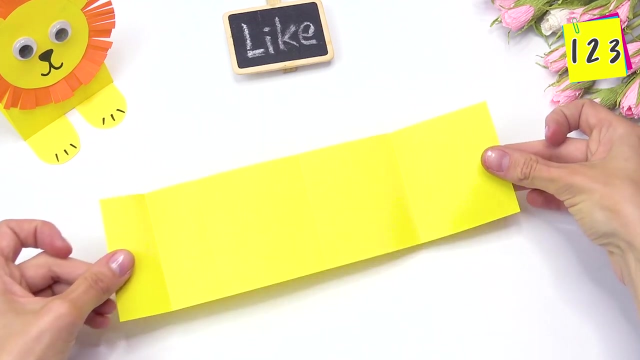 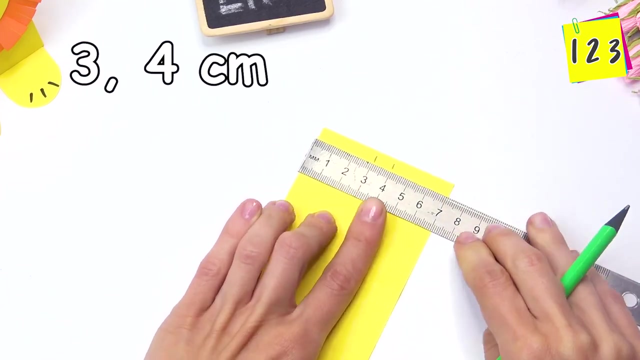 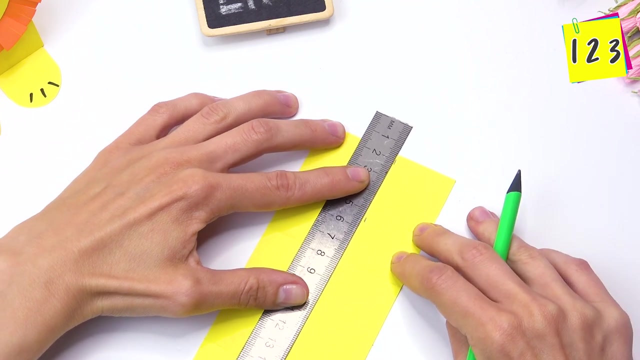 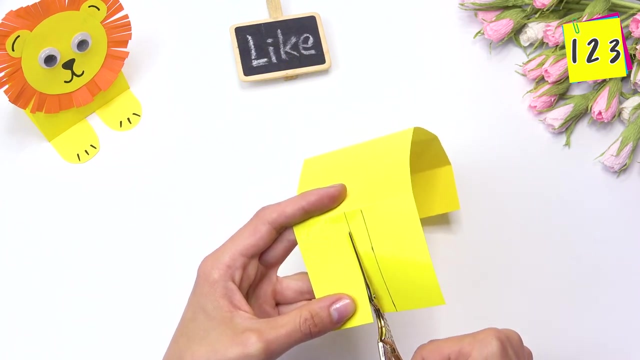 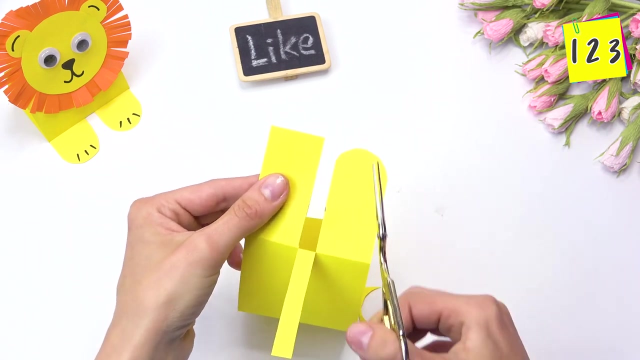 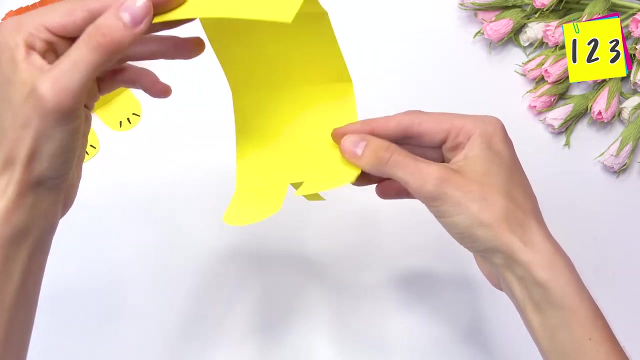 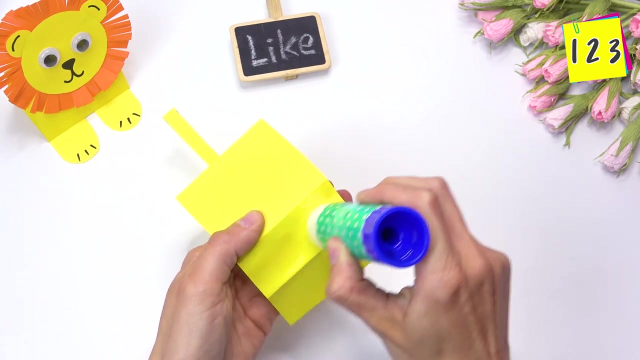 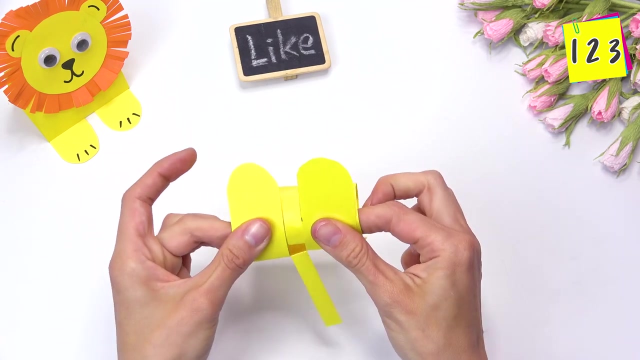 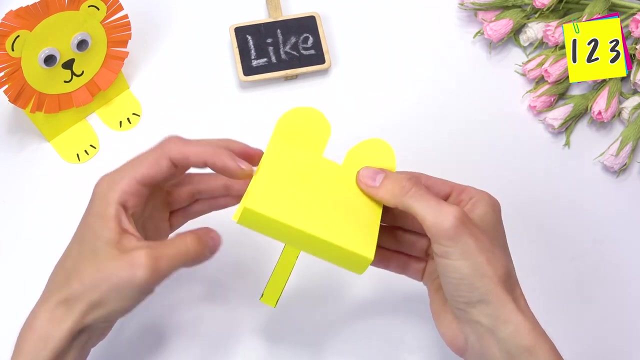 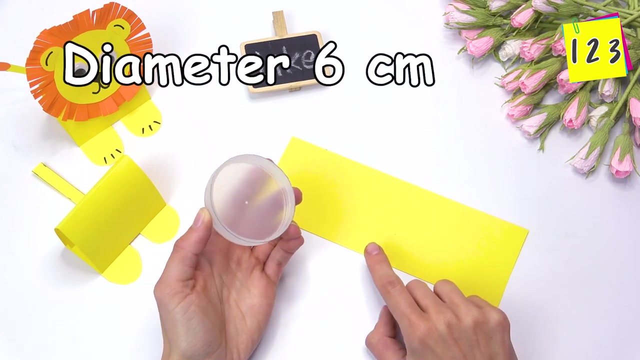 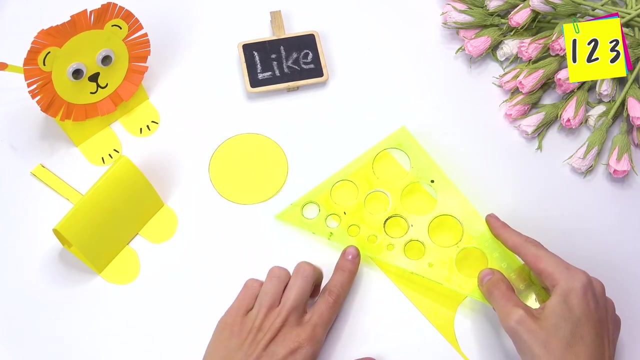 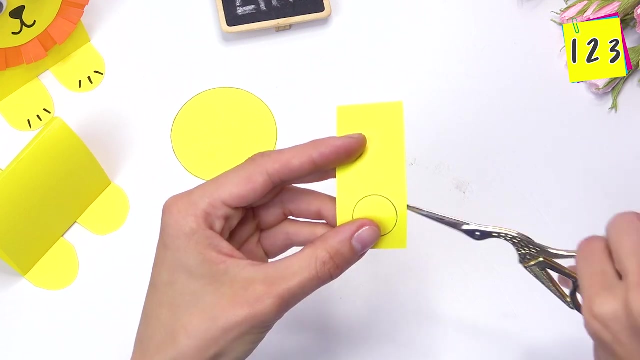 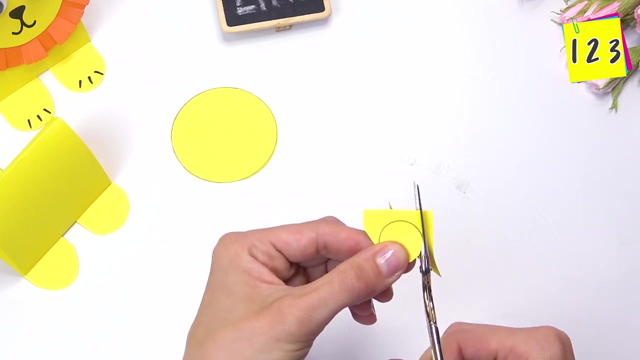 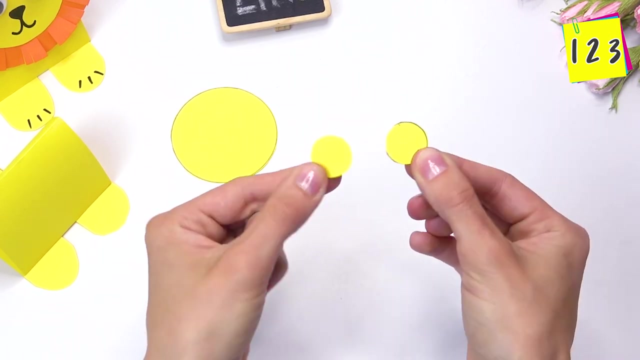 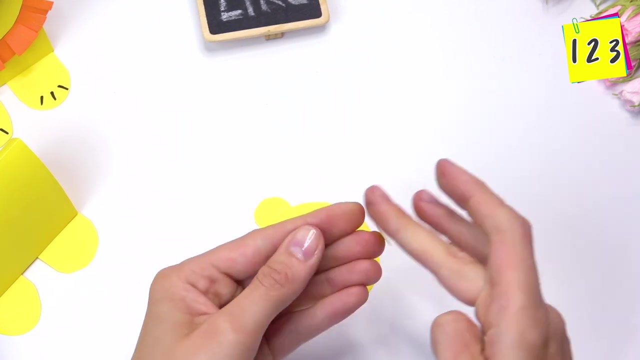 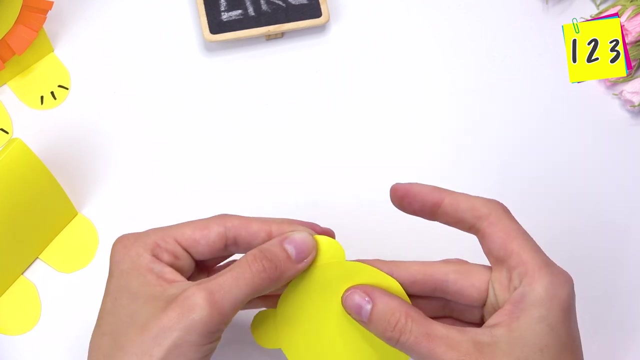 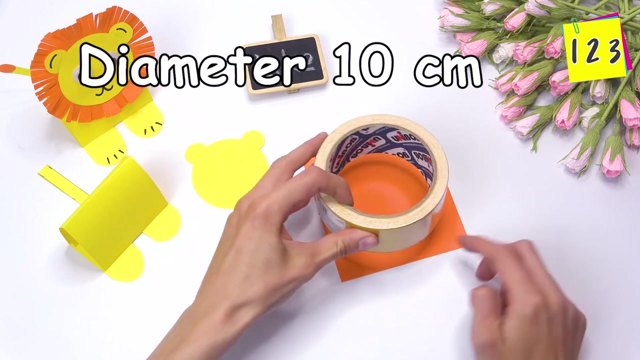 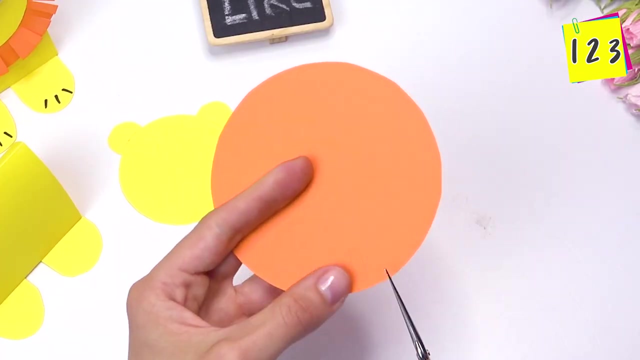 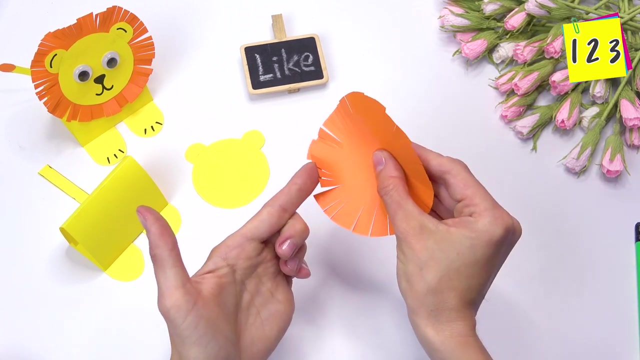 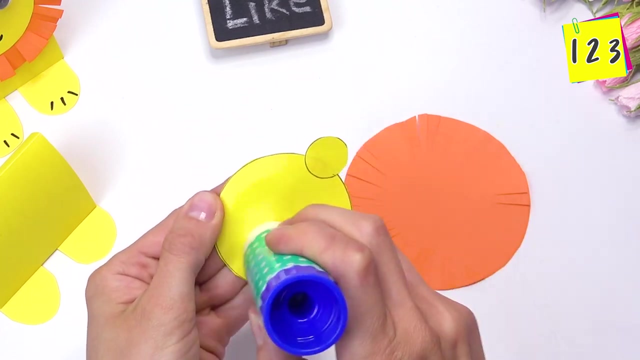 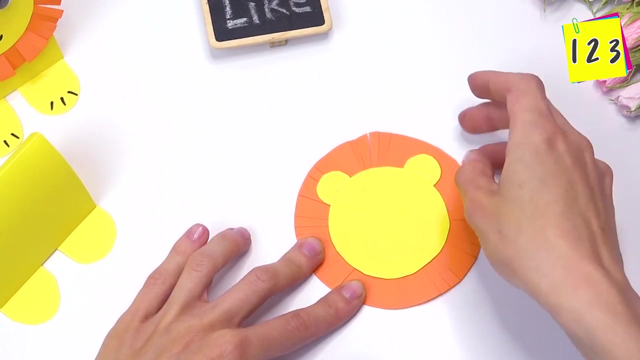 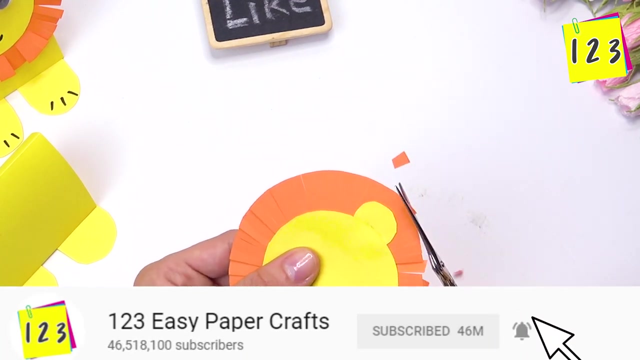 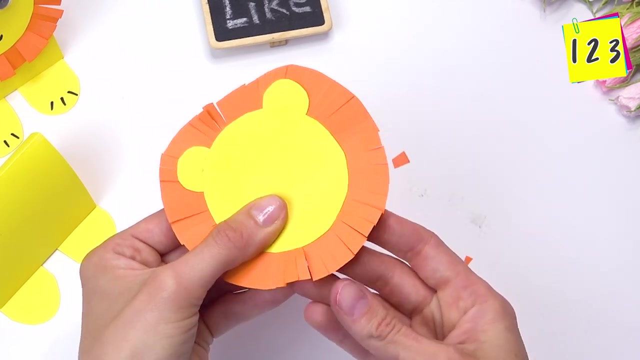 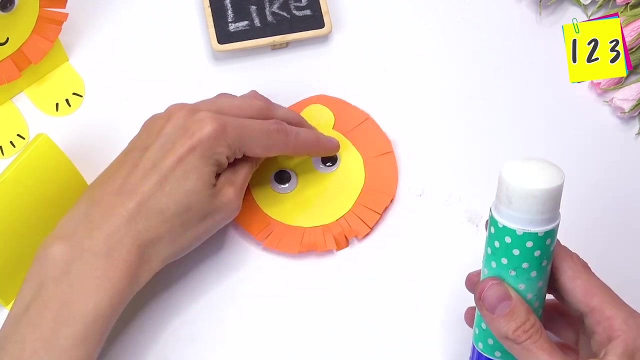 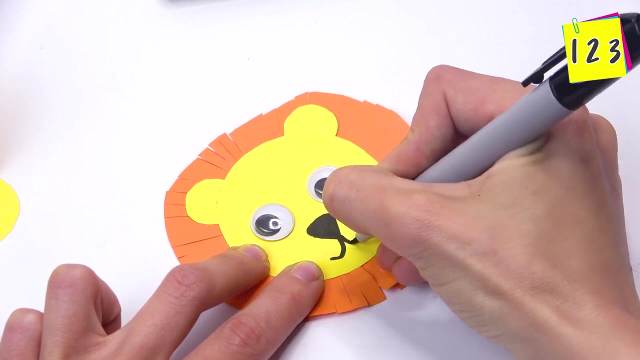 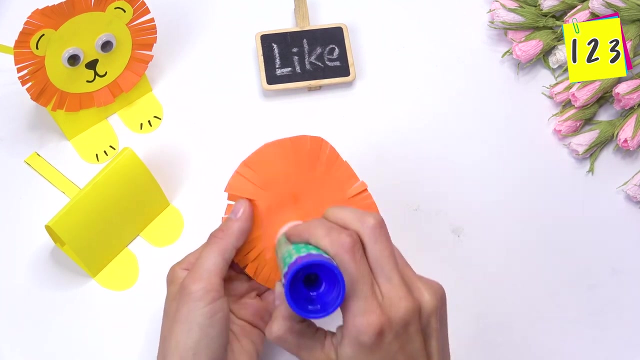 One, two, three Easy paper crafts. April Fools Face. The day has come for three things. April Fools face. I'll see you next time. Bye-bye, Bye-bye, Bye-bye, Bye-bye, Bye-bye.